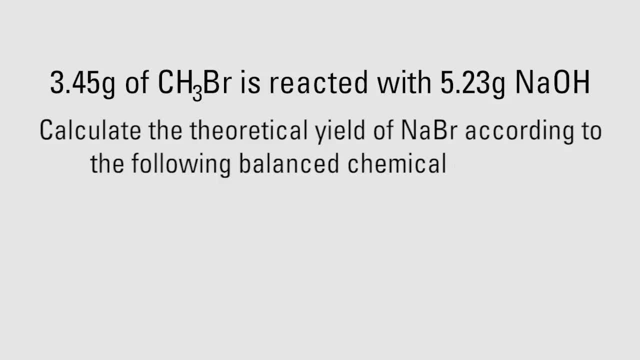 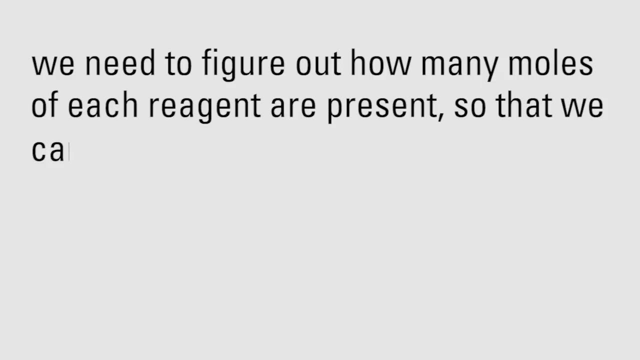 yield of sodium bromide according to the following balanced chemical equation: Methyl bromide plus sodium hydroxide yields methanol plus sodium bromide. We need to figure out how many moles of each reagent are present so that we can find the 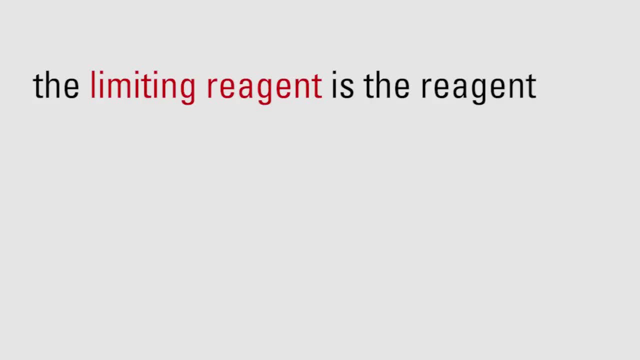 limiting reagent. The limiting reagent is the reagent that will be used to find the limiting reagent. The limiting reagent is the reagent that will be used to find the limiting reagent, The limiting used up completely, thus limiting the extent of the reaction. 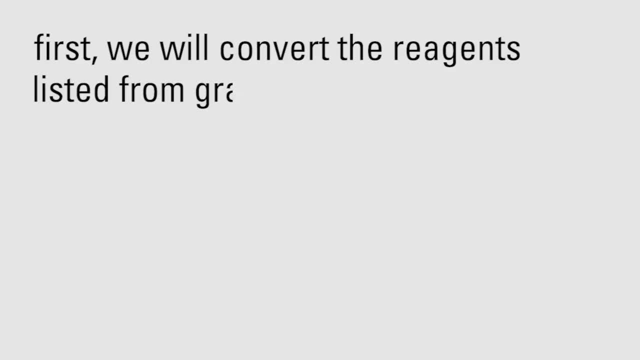 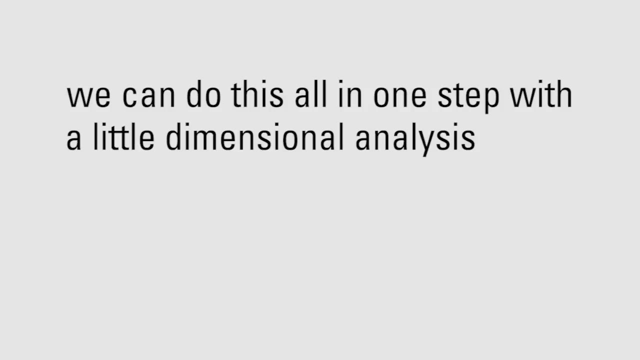 First we will convert the reagents listed from grams to moles. Next we will find how many moles of product we can form with our calculated moles of reagent. We can do this all in one step with a little dimensional analysis. 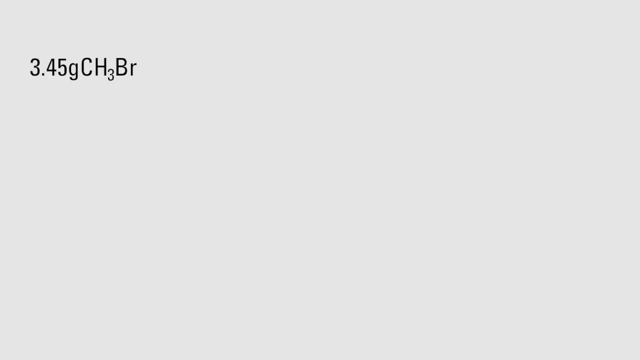 Multiply 3.45 grams of methyl bromide times 1 over the molar mass, or 1 mole of methyl bromide over 94.94 grams of methyl bromide. Then multiply by the ratio of sodium bromide to methyl bromide. 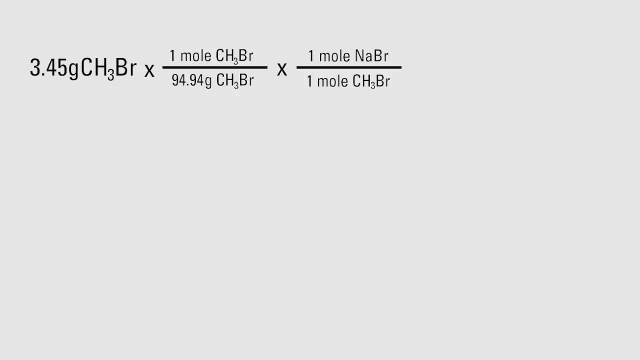 reaction coefficients, which is 1 to 1.. This gives us 0.0363 moles of sodium bromide. Now we will do the same for sodium hydroxide. Multiply 5.23 grams of sodium hydroxide times 1 over the molar mass. 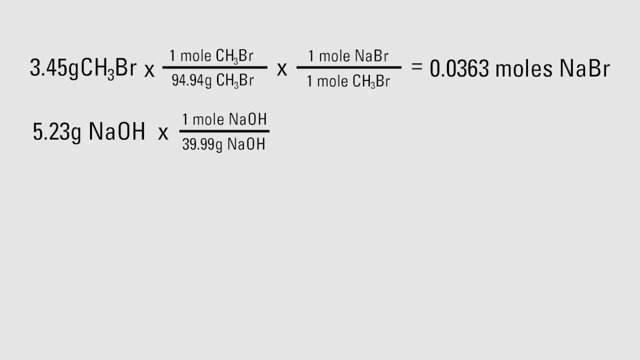 or 1 mole of sodium hydroxide over 39.99 grams of sodium hydroxide. Then multiply by the ratio of sodium bromide to sodium hydroxide reaction coefficients, which is 1 to 1.. It is very important to make sure that you use the proper reaction coefficients. 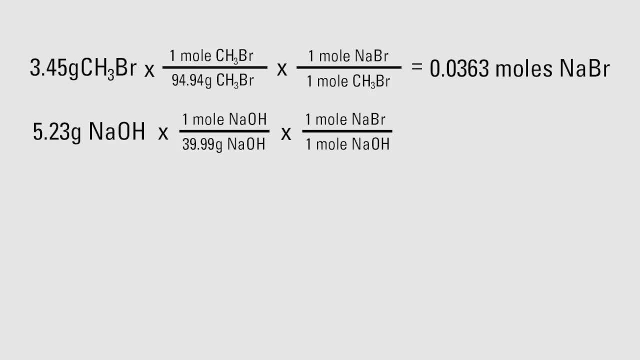 This example is simple and at the rate of 1,, the ratio is 1 to 1.. Nevertheless, this step is important. This calculation gives us 0.1308 moles of sodium bromide. We can see that the 3.45 grams of methyl bromide 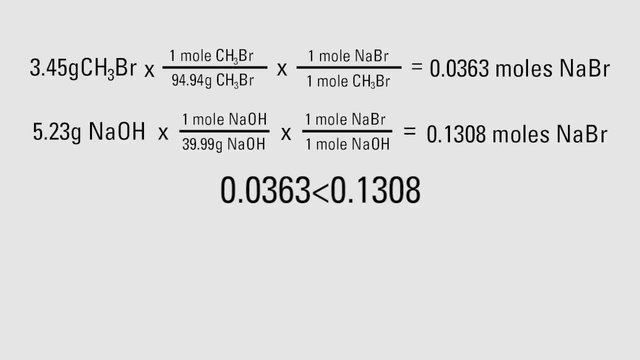 is going to produce less moles of bromide than hydroxide, and thus all of the methyl bromide will react completely. Therefore, methyl bromide is our limiting reagent. Theoretical yield tells us how much product we should end up with.